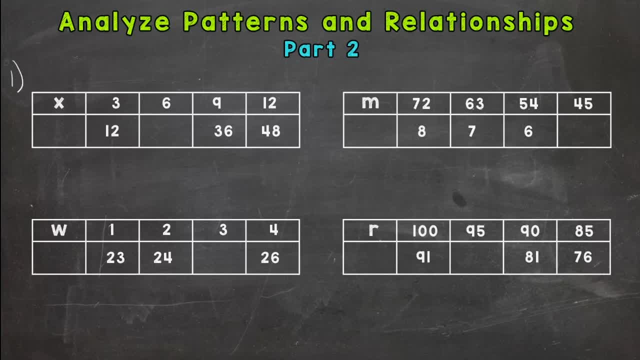 So let's look at number 1 here with the X, and I'll number these 1, and we'll go to the side for number 2, 3, and 4.. So we have a table here. We're going to write in a rule here for the corresponding terms. 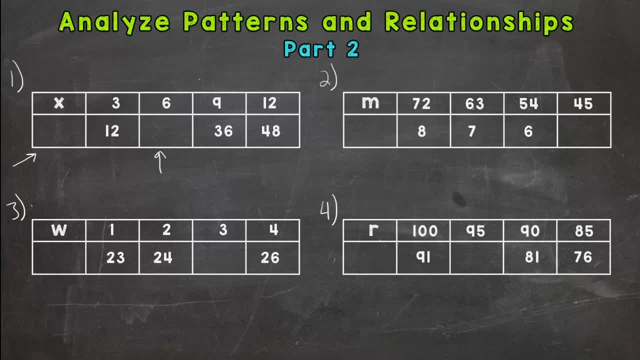 And then we have a missing term In the pattern that goes there. So along the top right here we have 3, 6, 9,, 12.. So counting up by 3's, Let's check for our relationship between corresponding terms. 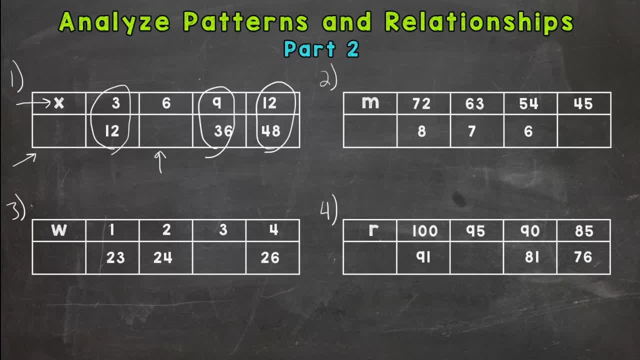 Remember corresponding terms are the matching pairs between the two patterns, basically the partners, So 3 and 12.. 9 and 36,, 12 and 48. And then, Once we find the relationship, that can help us find the missing piece. that goes right there. 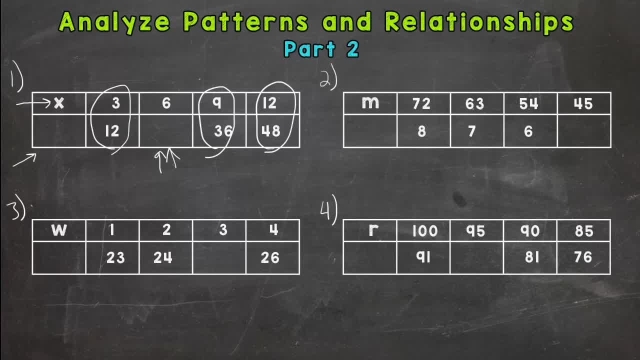 So how do we get 3 equal 12?? We're increasing in value, so it's either going to be addition or multiplication. Let's try add 9.. 3 plus 9 does equal 12.. Let's try it for 9 to 36.. 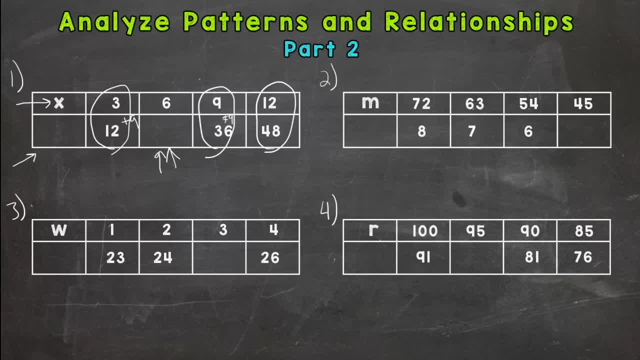 9 plus 9, does that give us 36?? No, So adding 9. Does not work. Remember it has to work for all of them. Think of a multiplication fact: How do I get 3 to equal 12?? 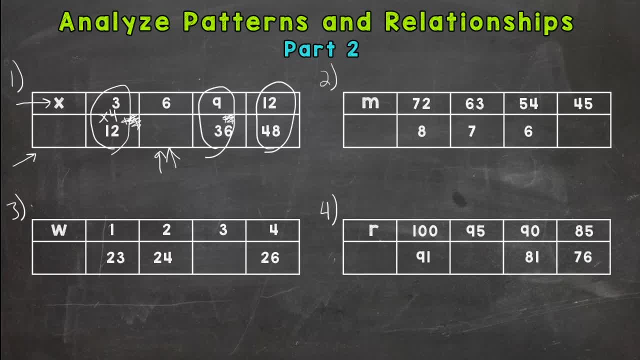 Hopefully you're thinking multiply by 4.. 3 times 4 is 12.. 9 times 4 is 36.. And 12 times 4 is 48. Let's apply it to our 6 here: 6 times 4 is 24.. 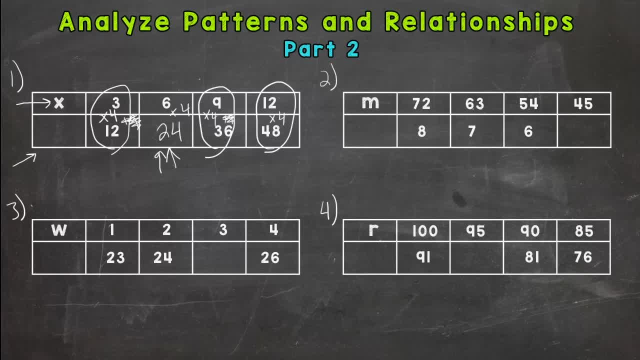 So that's our missing piece. And then our rule is: We're multiplying x by 4.. Remember, a number next to a letter means multiply. So our rule for how to get our top terms to equal our bottom terms is we multiply our x's up here by 4 to get the corresponding term below. 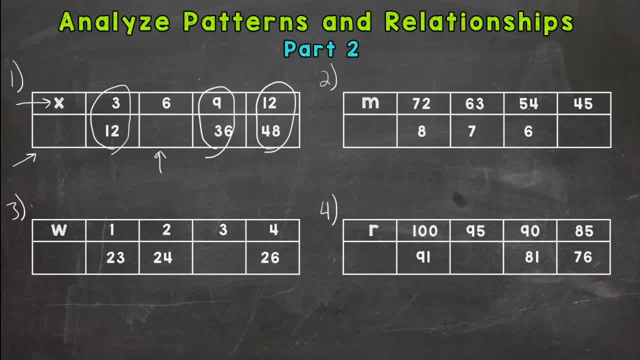 Remember corresponding terms are the matching pairs between the two patterns, basically the partners, So 3 and 12.. 9 and 36,, 12 and 48. And then, Once we find the relationship, that can help us find the missing piece. that goes right there. 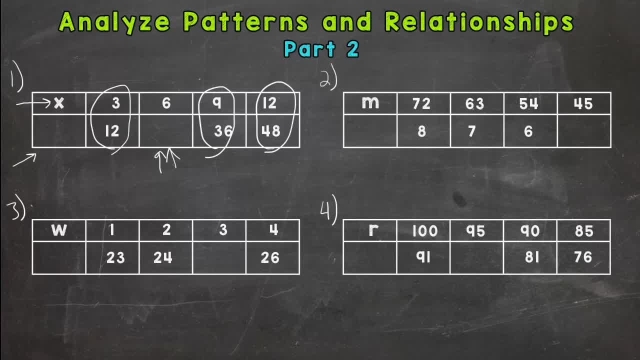 So how do we get 3 equals 12?? We're increasing in value, so it's either going to be addition or multiplication. Let's try add 9.. 3 plus 9 does equal 12.. Let's try it for 9 to 36.. 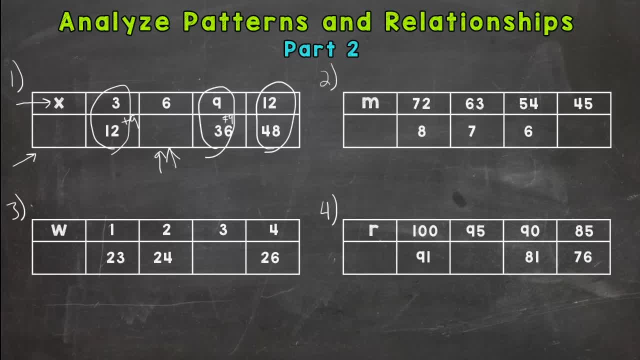 9 plus 9, does that give us 36?? No, So adding 9. Does not work. Remember it has to work for all of them. Think of a multiplication fact: How do I get 3 to equal 12?? 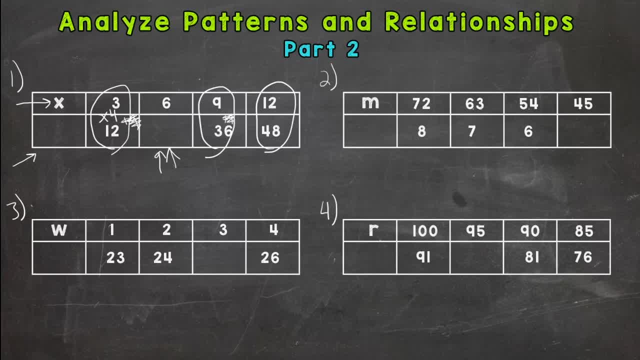 Hopefully you're thinking times by Multiply by 4.. 3 times 4 is 12.. 9 times 4 is 36.. And 12 times 4 is 48.. Let's apply it to our 6 here: 6 times 4 is 24.. 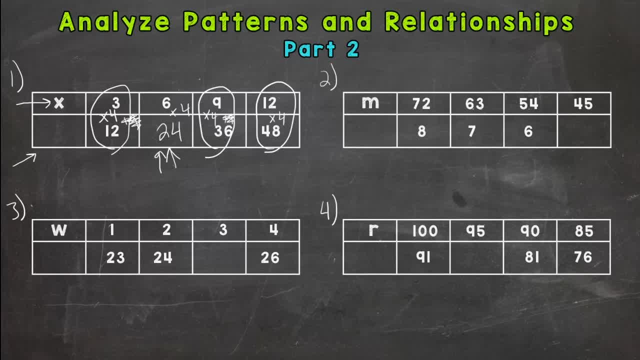 So that's our missing piece. And then our rule is: We're multiplying x by 4.. Remember, a number next to a letter means multiply. So our rule for how to get our top terms to equal our bottom terms is: we multiply our. 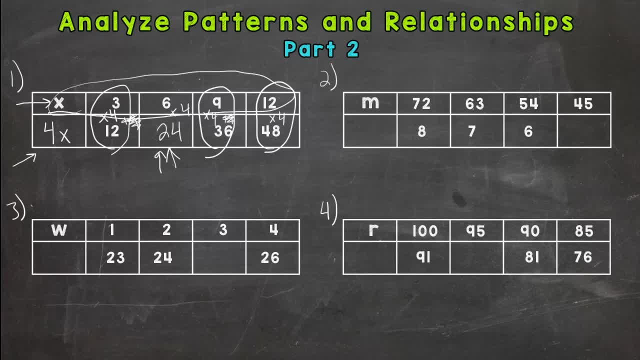 x's up here by 4 to get the corresponding term below. Let's go to number 2 here, 72 and 8,, corresponding terms 63 and 7,, 54 and 6, and then we have a missing term. 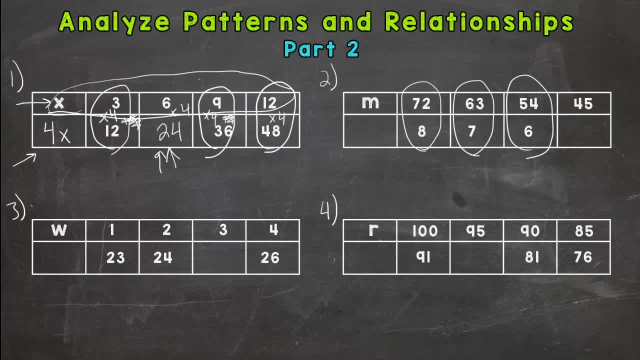 So 72 to equal 8.. We are decreasing in value, so it's going to be subtraction or division, And this is actually going to be: 72 divided by 9 equals 8.. Let's try it for the other ones: 63 divided by 9 does equal 7.. 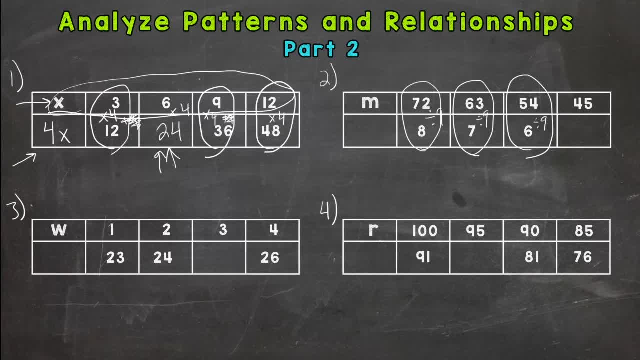 And 54 divided by 9 does equal 6.. So what's 45 divided by 9 going to give us 5.. Now you may have been able to figure that number out by going 8,, 7,, 6,, 5.. 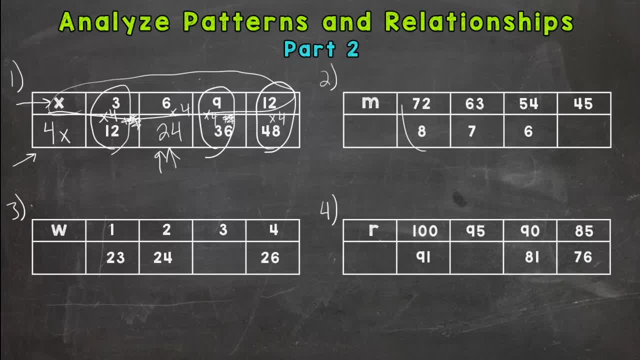 Let's go to number 2 here: 72 and 8, corresponding terms 63 and 7,, 54 and 6.. And then we have a missing term. So 72 to equal 8. we are decreasing in value. so it's going to be subtraction or division. 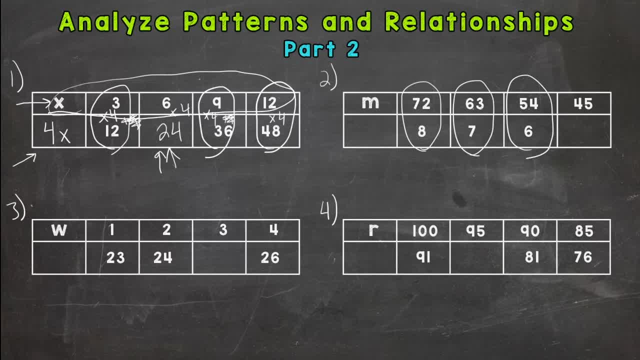 and this is actually going to be: 72 divided by 9 equals 8. let's try for the other ones: 63 divided by 9 does equal 7, and 54 divided by 9 does equal 6. so what's 45 divided by 9 going to? 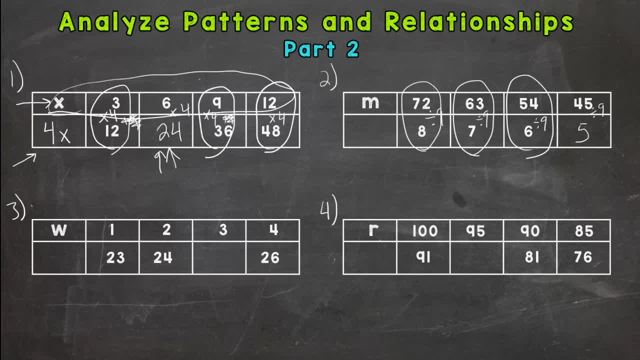 give us 5. now you may have been able to figure that number out by going 8, 7, 6, 5. that's fine if you follow the bottom pattern to figure that out, but always make sure your rule applies. double check with the 45 divided by 9 does give me the 5, and our rule is we are taking m and dividing it. 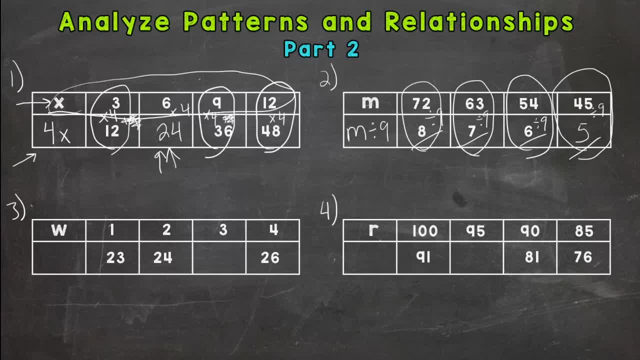 by 9 to give us our corresponding term below. let's go to number 3. how do we get 1 to equal 23, 2 to equal 24- we have a missing piece- and then 4 to equal 26, so it's either going to be addition or multiplication, because we're going up. 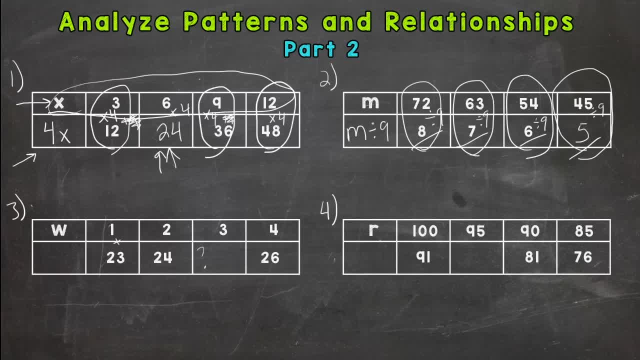 in value. let's try addition. what can we add to 1 to give us 23? hopefully you're thinking 22. let's see if it works. 1 plus 22 is 23. it works for these corresponding terms: 2 plus 22 does equal 24. and then 4 plus 22 does give us 26. 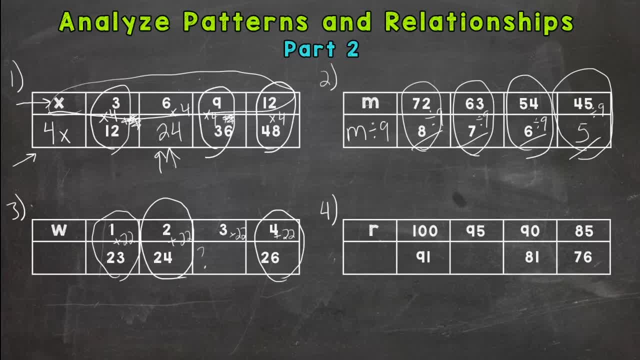 so let's apply our rule to our missing piece here. 3 plus 22 does give us 25 for our missing piece, and our rule is: w plus 22 gives us our corresponding terms below. so if we take these W's and we add 22, we get the numbers below all. 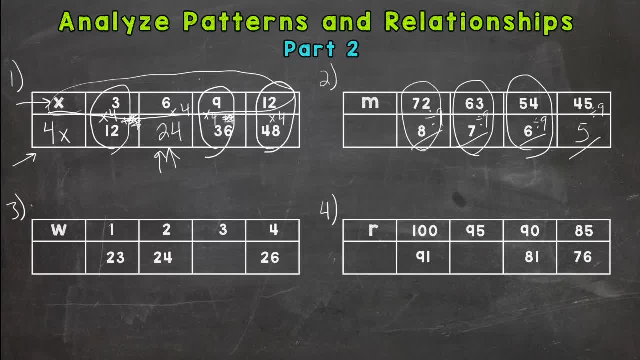 That's fine if you follow the bottom pattern to figure that out, But always make sure your rule applies. Double check with the 45 divided by 9 does give me the 5. And our rule is we are taking m and dividing it by 9 to give us our corresponding terms below. 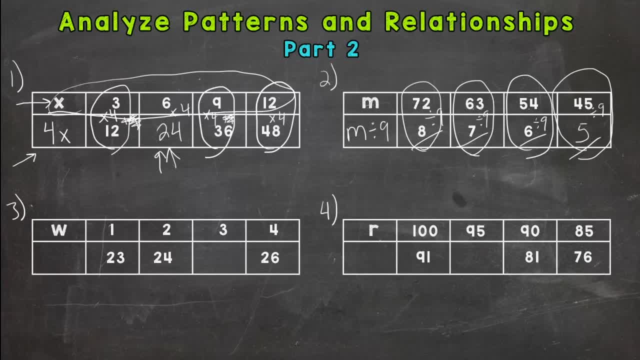 Let's go to number 3.. How do we get 1 to equal 23,, 2 to equal 24? We have a missing piece, And then 4 to equal 26. So it's either going to be addition or multiplication, because we're going up in value. 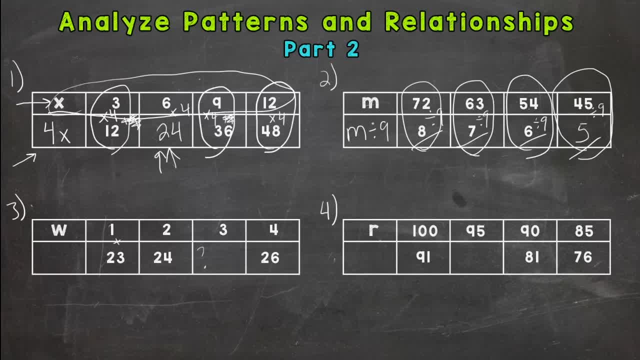 Let's try addition. What can we add to 1 to give us 23?? Hopefully you're thinking 22.. Let's see if it works. 1 plus 22 is 23.. It works. It works for these corresponding terms. 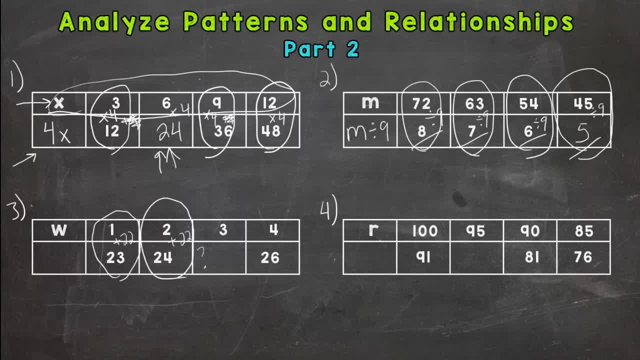 2 plus 22 does equal 24.. And then 4 plus 22 does give us 26.. So let's apply our rule to our missing piece here: 3 plus 22 does give us 25 for our missing piece, And our rule is: w plus 22 gives us our corresponding terms. 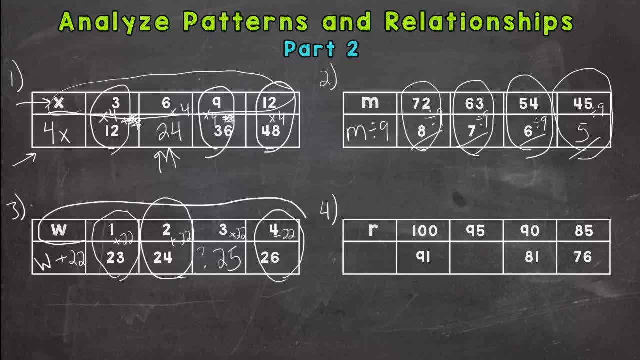 So if we take these w's and we add 22, we get the numbers below. Alright, then number 4.. 195, 90, 85 looks like we're counting down by 5. And we have 100 to equal 91, so we're decreasing in value. 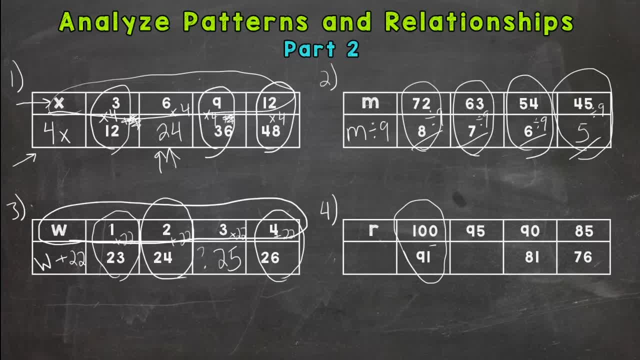 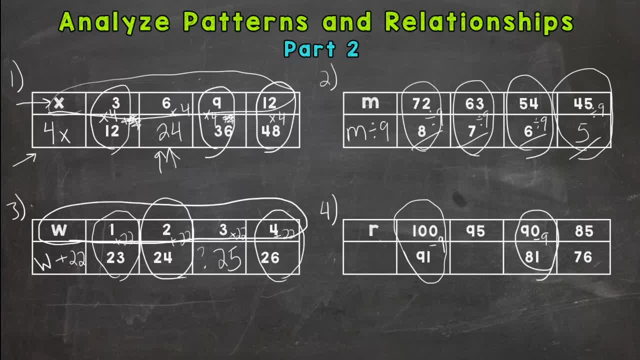